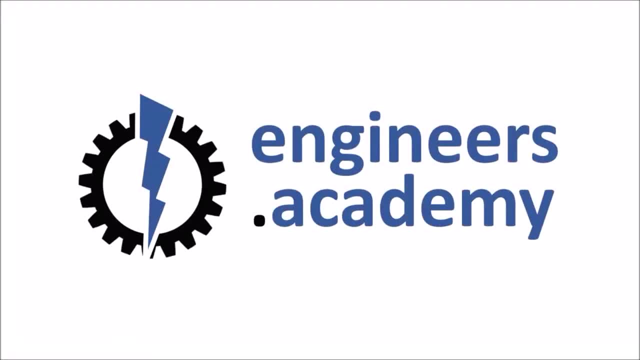 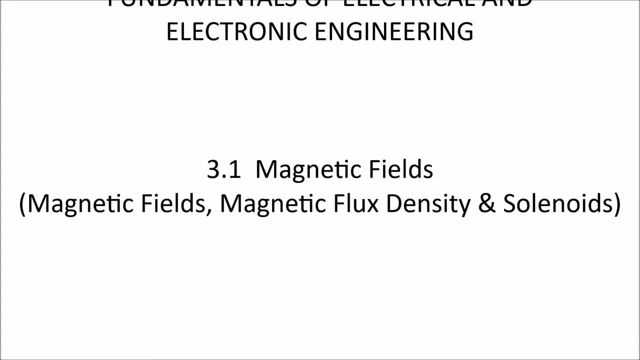 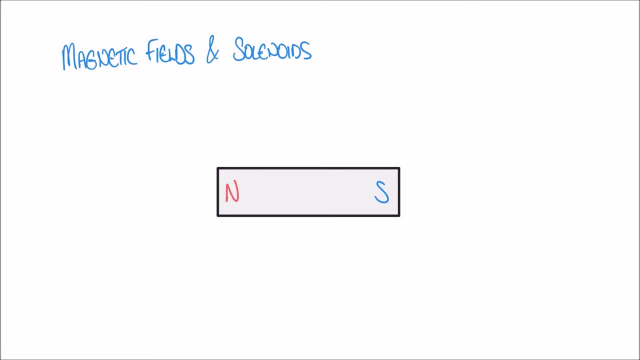 In this video we're going to expand on what we looked at in our previous video on electromagnetic fields and we're going to look at magnetic fields in a bit more detail and we're also going to look at solenoids which are an example of an electromagnet. But before we get on to that I want to look at even just the most basic magnet, a bar magnet like the one in the diagram below. We know that a magnet obviously has magnetic properties and we can represent those magnetic properties by a magnetic field and the way we draw a magnetic field for a bar magnet is by drawing field lines that travel from the north to the south pole and so we can draw them on something like this. We have lines that travel from the north to the south pole like so and a few properties of these field lines are firstly that they have a direction and so we said that the field lines are going from north to south and so we should make that clear on our diagram. Another thing that should be true for our field diagram is that because the field gets weaker as we get further from the magnet the spacing between the field lines should get bigger which isn't necessarily perfectly the case for my diagram but I've done my best here. So the spacing should get wider and wider as we get further from the magnet and that's meant to represent 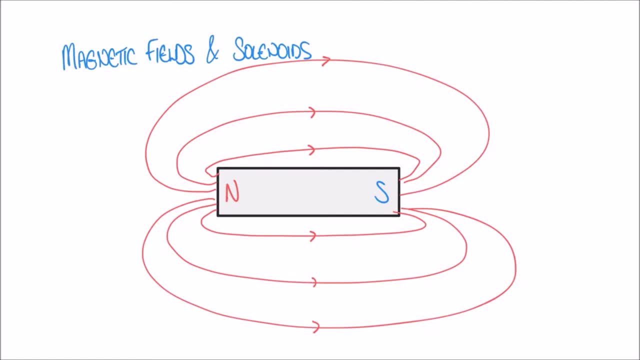 the magnetic field getting weaker as we get further from the magnet. What we can also see from our 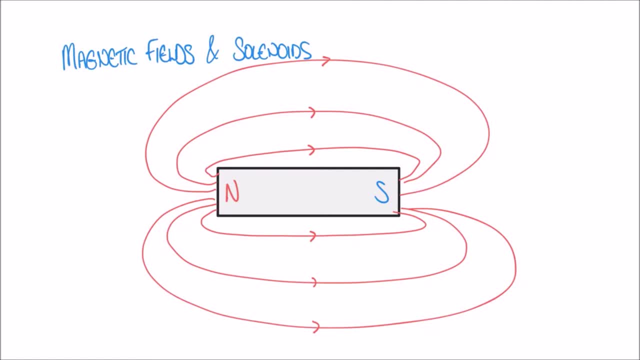 diagram here is if the closeness of the lines represents the strength of the magnetic field then the strongest magnetic field is going to be found near the poles of the magnet where these lines are the most concentrated, the most dense. So I want to mark a few things on our diagram here. 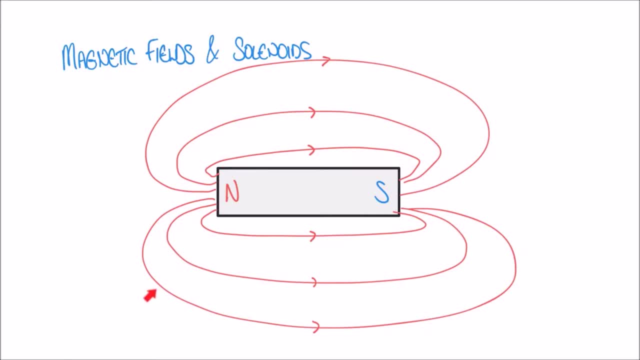 First of all the proper term for these these lines is something called magnetic flux and magnetic flux is represented by field lines but we can make a note of it here so magnetic flux is the proper term. 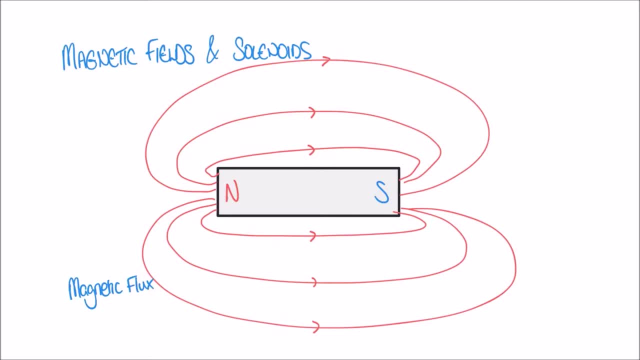 And usually we give magnetic flux the Greek letter Phi as its symbol which is almost like a capital I with a circle inside of it. And magnetic flux has a unit it's measured in Webers. 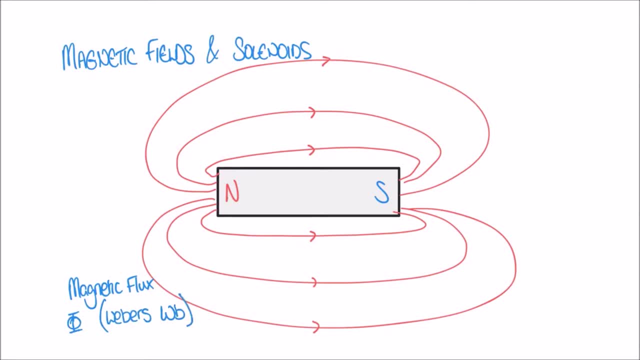 Often shorted shortened to just WB but we measure magnetic flux in Webers. 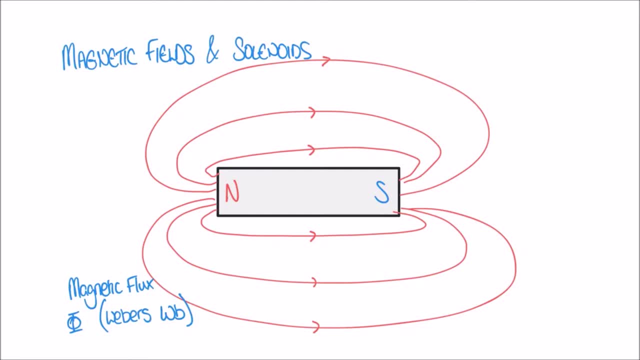 The next thing to think about on our diagram is area because we've mentioned that there are some areas of our of our diagram for instance when we're far away from the magnet where the field lines are quite sparse. So if we look at this diagram we can see that there are some areas of our of our diagram for instance when we're far away from the magnet where the field lines are quite sparse. Whereas there are some areas on the diagram where the field lines are quite compact and that obviously has some kind of implication on the strength of the magnetic field. and so what I want to do is I want to try and represent area on this diagram. If we imagine that we have an area for instance I'll try and draw sort of 3d representation of an area and I'll call it A. 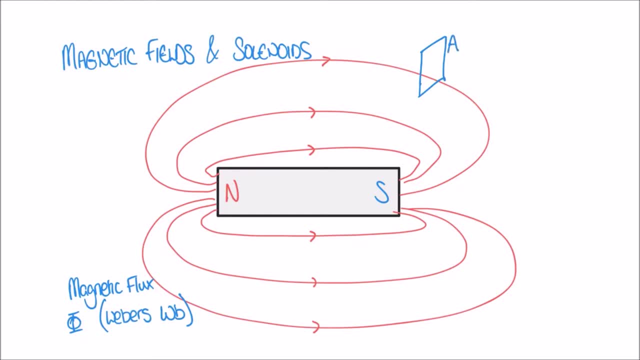 Well this this particular area that I've drawn has only one area. only one field line going through it whereas if I draw the same sort of area if even if I imagine it's the end of our bar magnet I can try and represent the area of the end of the bar magnet there and we can see that there are one two three four five six lines of magnetic flux going through that area there and so the area has an implication on something called the magnetic flux density and magnetic flux density we give the letter B and the formula for B the magnetic flux density is simply Phi over A so it's the magnetic flux divided by the area so for instance in our top area here we have very little magnetic flux and we have very little magnetic flux so it's the magnetic flux divided by the area so it's the magnetic flux going through a given area and so B the magnetic flux density is going to be very low whereas in a different area I have quite a high magnetic flux divided by roughly the same area and so the magnetic flux density is going to be high in this instance so I could mark on my diagram here that this is a an example of low B 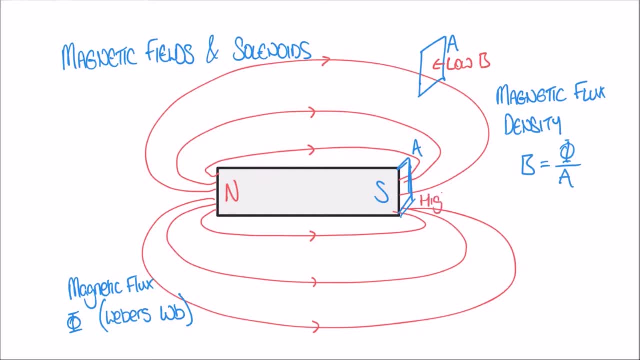 and this is an example of high B high flux density let's have a go at trying to work out the magnetic flux density at the end of this magnet here and let's see that we know that the magnetic flux in this instance is five hundred microwebers so I'll make a note of that and we'll see that Phi is five hundred microwebers 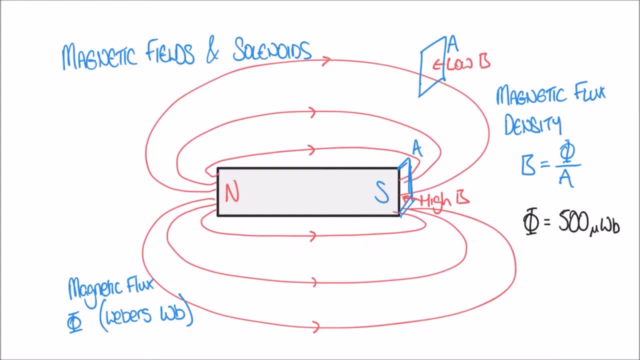 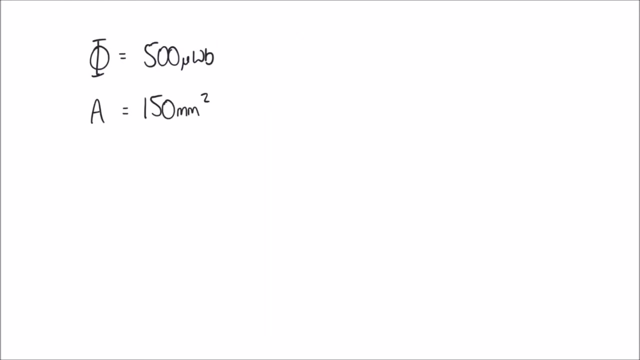 and let's say that we know that the area of the end of this magnet is 150 millimeters squared so 150 square millimeters is our area and what we want to try and do now is work out the magnetic flux density of this area here at the end of the magnet so to calculate this we're going to use our formula b equals phi over a and in this case we 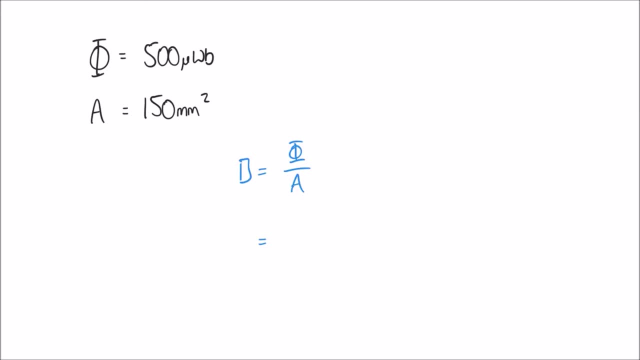 know that phi is 500 micro webers now we know our standard prefix micro represents 10 to the minus six so in our formula we should say 500 times 10 to the minus six webers over the area we're going to use our formula b equals phi over a and in this case we know that phi is 500 micro which is given in millimeters squared now our si unit is meters something to be careful of here is that although there are a thousand millimeters in a meter there are a million millimeters squared in a meter squared because if we think of a meter we have imagine a meter squared 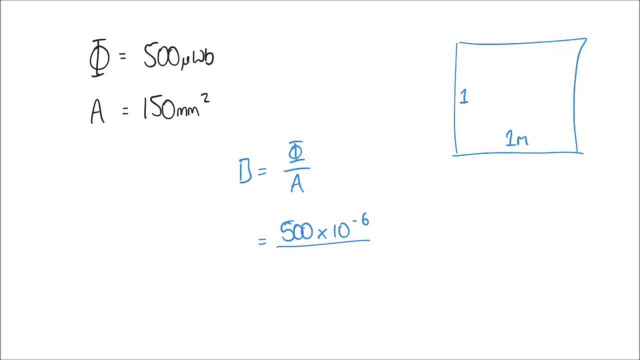 one meter by one meter there are a thousand me. 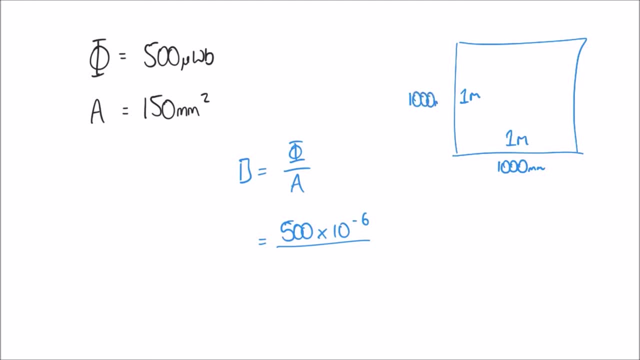 millimeters by a thousand millimeters along the side so that gives us a total of a million square millimeters if we multiply them together and so we've got to be careful when we're converting our area 150 millimeters squared into meters squared so because there's a million millimeters 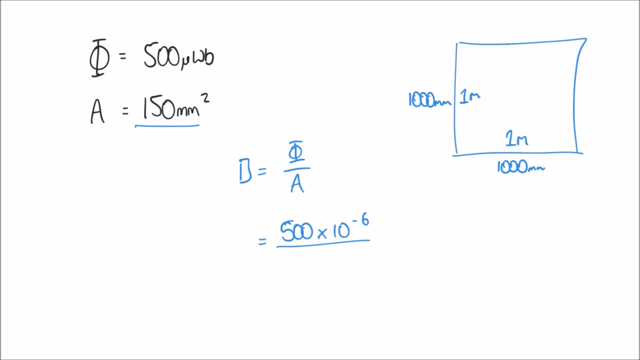 squared in a meter squared we have to use the 10 to the minus 6 in this instance as well for a millionth so we'll say 150 times 10 to the minus 6 and if we cancel those 10 to the minus 6 is out because we've got a 10 to the minus 6 on the top and on the bottom there we're left with 500 over 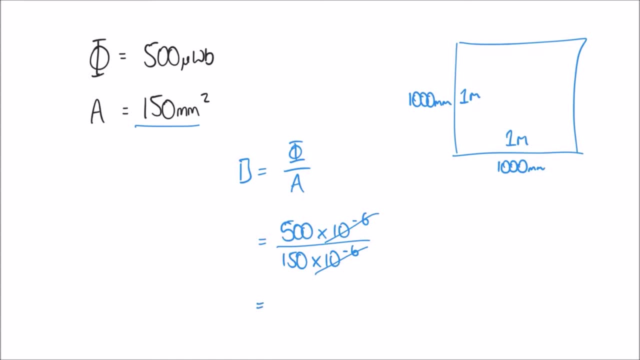 150 which gives us 3.33 3.33 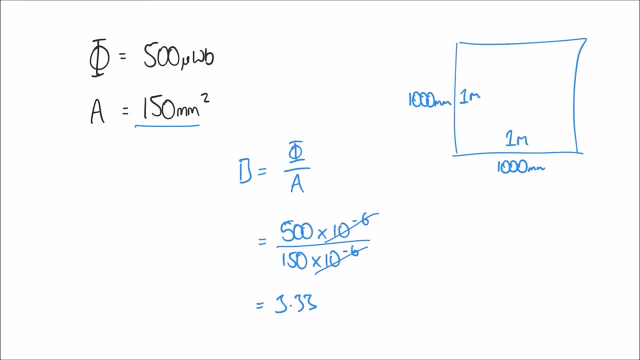 finally the unit of magnetic flux density is tesla so we give it the capital t for tesla so b is magnetic flux density 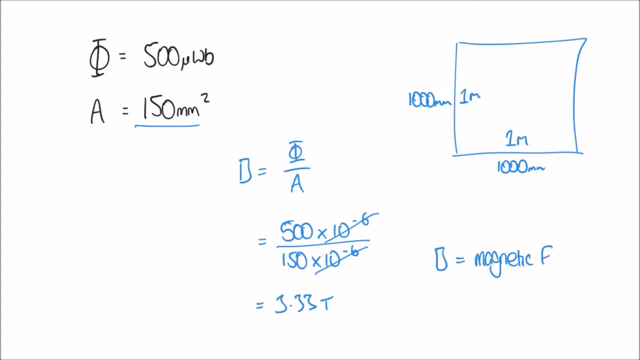 and it's measured in tesla t-e-s-l-a or just a capital t for short 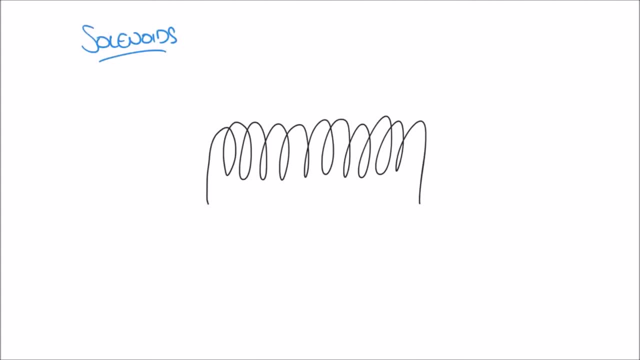 and it's actually actually a small t which is just to put it like that 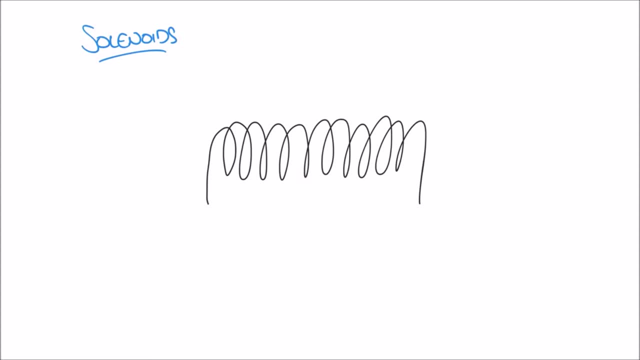 in a previous video we've talked about how a conducting wire produces a magnetic field when 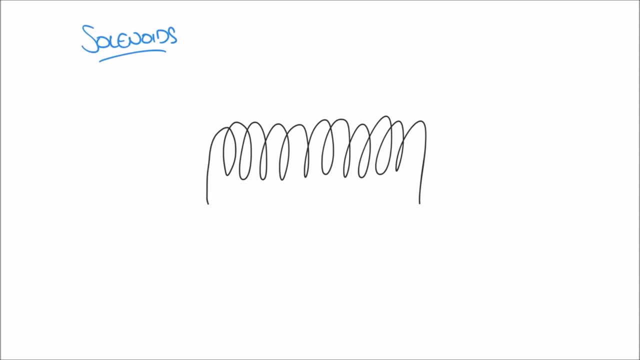 a current flows through it and what we can do is we can take advantage of that by coiling a wire into what's called a solenoid and what we find is that when we have a coil of wire like the one in the diagram here and we pass a current through that wire we see themomentum istoclub so opetite equal to obtained current real magnet общемon! 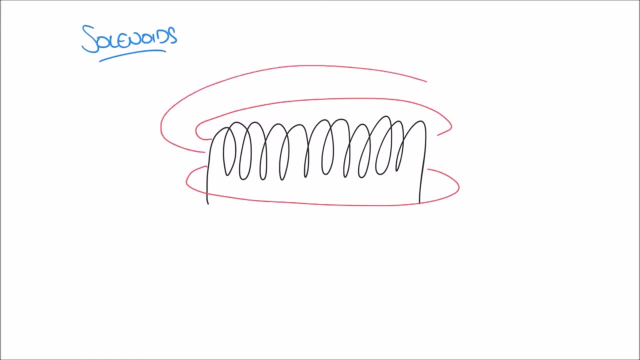 the same sort of shape through the wire itself we see that which is called the piece which is located in the process ofidir Alex theなく we see the same sort type of shape of wire as both this one app Ahmed Kemald putty magnetic field as we would see in a bar magnet and so we get a magnetic field 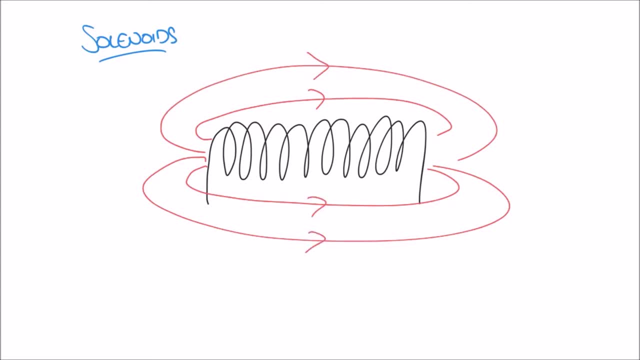 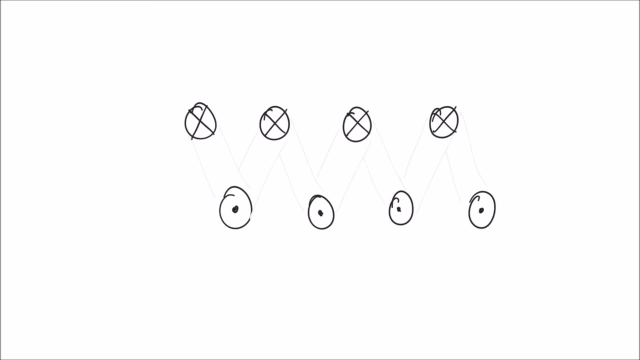 produced let's have a closer look as to why that's the case in our previous video we looked at the symbols for conductors with currents traveling away from us and currents traveling towards us and what we can imagine is if we kind of take a cross section of the coil that we've seen on the previous slide we might see something like this and what we have is along the top there conductors with currents traveling away from us and then looping back around along the bottom there we have those currents traveling back towards us again and so we can think of a coil as a combination of these currents traveling away and towards us and what we spoke about in the last video is that currents traveling away from us produce a clockwise magnetic field and so what we can draw on here is magnetic fields i could 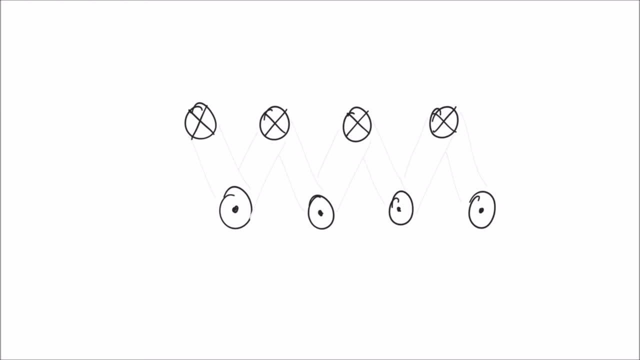 draw them individually around each conductor but what we talked about is that these magnetic fields sort of group together and so what we'll see is something that looks like this where we have a magnetic field produced and it's in a clockwise direction in the case of a current traveling away from us and so what we have is along the top here we have a magnetic field produced in that clockwise direction and along the bottom here we have a magnetic field produced in an anti-clockwise direction and what we can see is if we kind of expand on this this idea we'll see that we have this kind of similar magnetic field produced as a result of the behaviors of these two sets of conductors based on this we can calculate a new parameter which is called h the magnetic field strength and it's measured in this unit at the end here amp turns per meter which will become a little bit more apparent in just a second when we look at the formula so h is a measure of the strength of the magnetic field produced by the solenoid and we can say that h is calculated by the formula i n over l now in this case i is the carried by the solenoid the coil and we measure that in amps n is the number of turns of the coil and finally l is something called the length of the flux path now in the case of